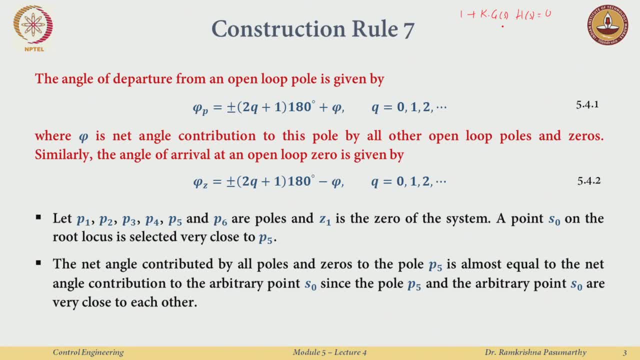 just that you know the magnitude criterion and the angle criterion. as simple as that. ok, So the angle of departure is given by, again, this angle criterion. So this is a little modification of that plus phi. ok, What is what is phi Say? I am interested in some pole. 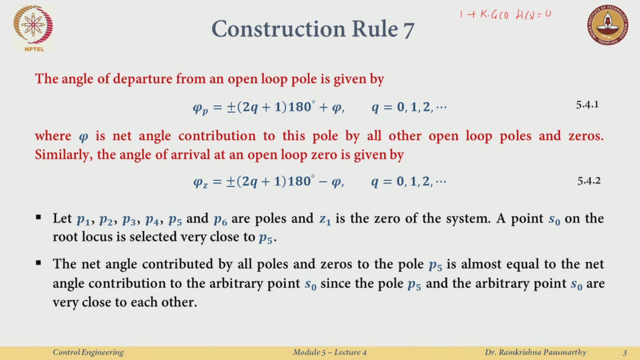 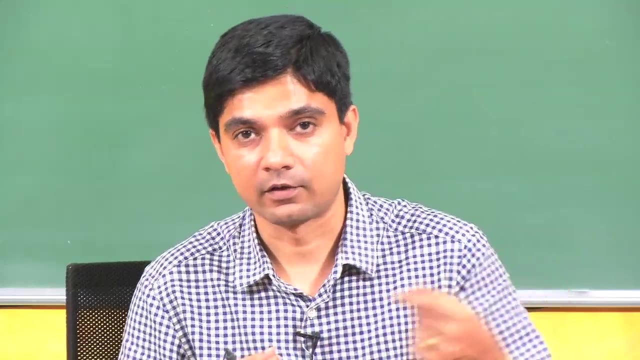 and this phi is the net angle contribution to this pole by all other open loop poles and zeros. ok, Now this is for pole right. I go away from a pole and then I end up at a 0. So I arrive at a 0. So which direction do I? do I arrive along the axis, or do I just? 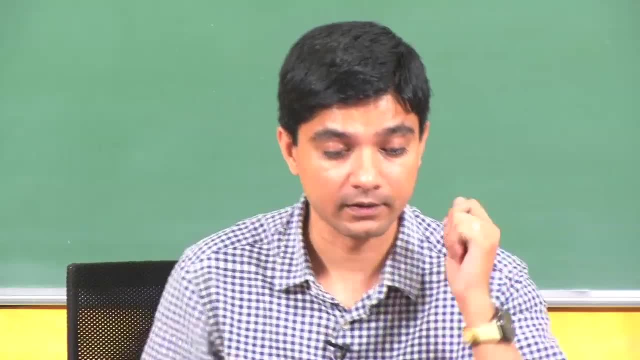 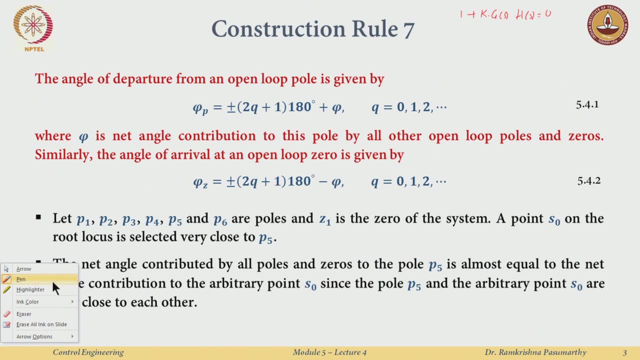 do some circular behavior or whatever. how do I arrive? that is also important, right? So the angle at arrival is again defined similarly. ok. So let us try to understand what this means. hence I draw a little picture here. So let us say I have 6 poles and 1, 0 and I am interested of you know how does p 5 move? ok, So let 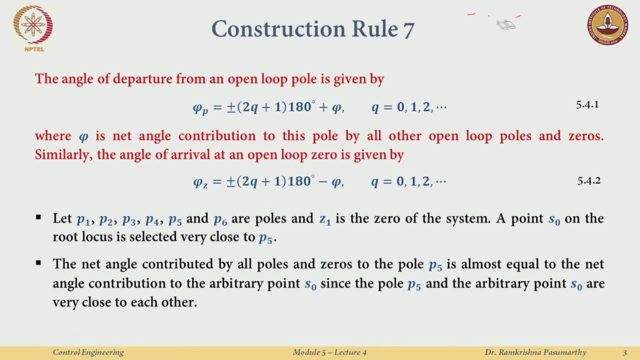 us get a little scenario here. ok, Let us get rid of this. ok. So 1 and p 5 becomes 1 and 0, right? So what I am doing is I am just defining here. So what do I do? I do a little standing. 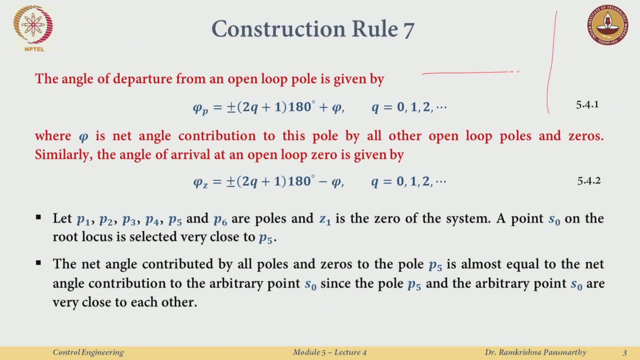 right, I am just some kind of things, So I am just trying to get the right angles right. So this is my plane and say, well, I have, we call this P 1,. I have P 2,, P 3,, P 4 and say 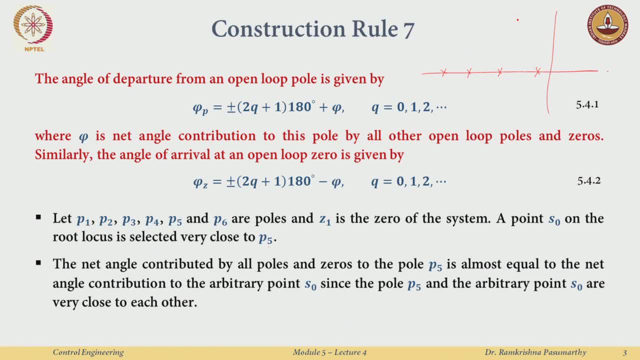 I have say P 5 and P 6 be here P 1,, P 2,, P 3,, P 4,, P 5 and P 6, ok, And then there is a 0, right. So let us say that the 0 is sitting somewhere here. ok, Now I want to see which. 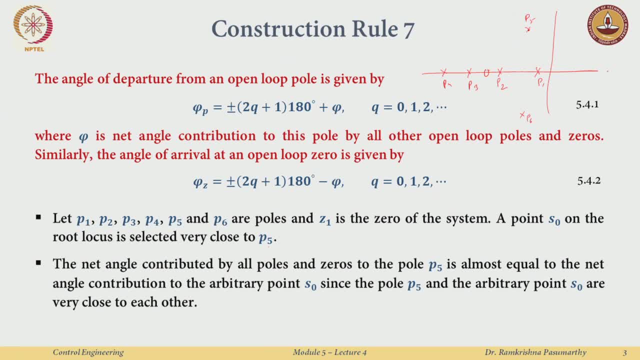 direction this guy should start moving. Should it start moving vertically downwards, or somewhere here or somewhere here for any arbitrary scenario? And let us say, I just take a point very close by here, this one, and I call that point as S naught. ok, Now for this S naught to lie on the root locus it. 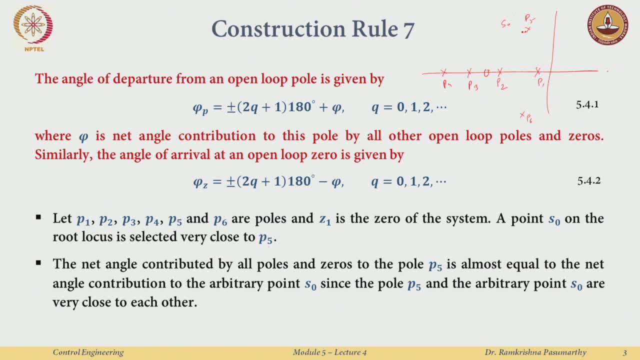 must for sure satisfy the angle criterion. ok, Now, and this is so which, this is just very close by right, So let us see. ok, So I just draw this. So these angles, this will be theta 4,, say theta 3,, I have theta 2,, I have theta 1, and 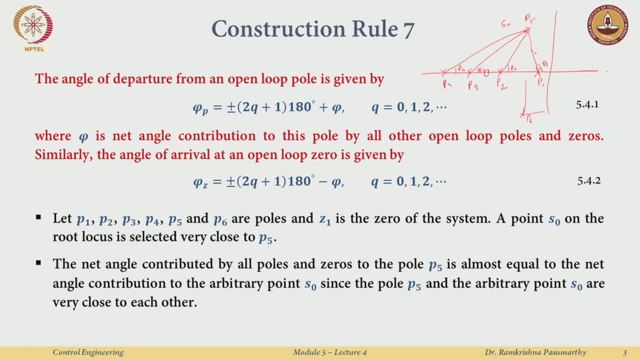 the angle here would be this guy, right? So some drawing this line from here, So that would be some theta 6 and then say: angle of this, of this: 0. I will just call this theta, ok. And then this guy is somewhere here, right? So? 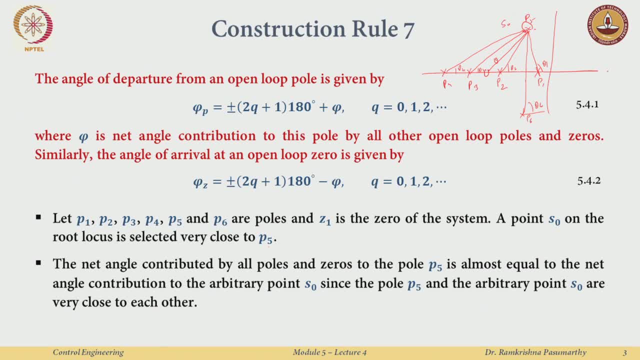 the angle here would be: So this guy is actually moving in this direction. ok, So this is the angle of theta p, right the pole which I am. I am interested in. ok, So here the phi's and theta's. but does not matter, right, you can just use whatever. ok? 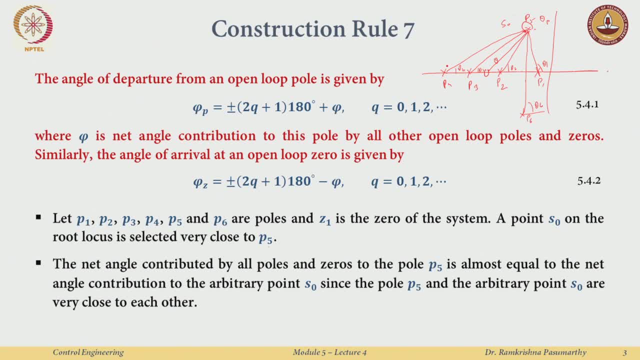 So for S 0 to lie on the pole. So what should happen? That all the sum of all these angles should again be multiples of 180 degrees. So what is? what is the? how is the angle criteria look like this: So what should happen? So, what should happen? So, what should happen? 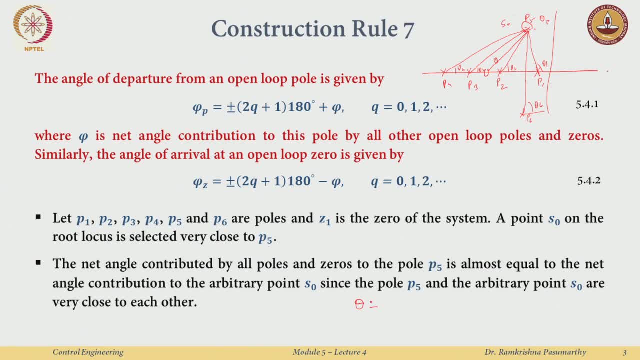 So this angle of the 0 is just theta, and then I have angle of all the poles, that is theta 1, theta 2, theta 3, theta 4, I have this little theta p, and theta 6 is again plus. 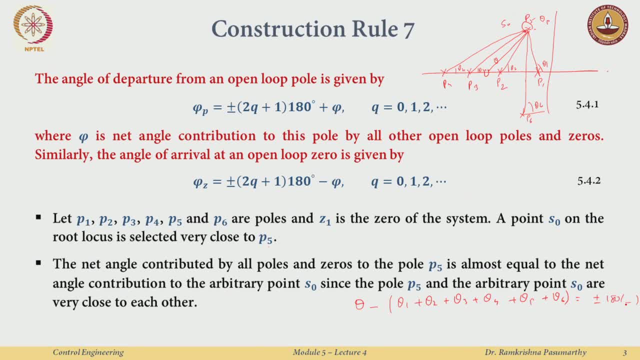 minus 180 and 2 q plus 1, blah, blah, blah. ok, Now I am interested in this angle, right, this guy, this little angle, This little angle, stare at theù, tell me where I will go. Therefore, I just, you know, substitute this and this theta. 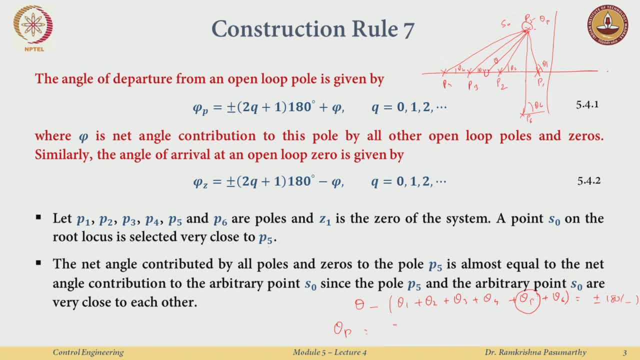 p or even phi. p, whatever is simply plus minus 2 q plus 1, 180 plus all the other remaining angles that just go here And I just call this sum from theta prime, right? So where, if this guy or this theta prime here, or ok, I just call this phi, this would be consistent. 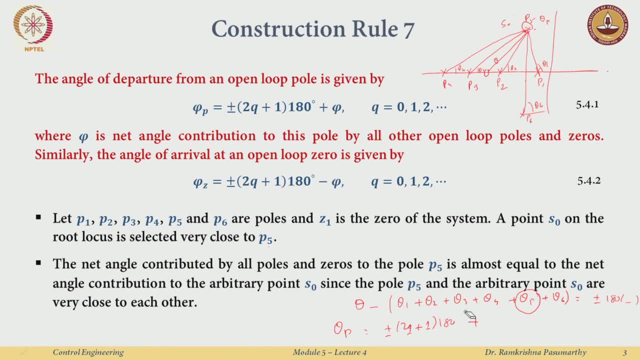 with brake notation over there. for all the others you can say: ok, So this phi is a net on angle contribution to this pole by all other open loop poles and 0s, right? So that is how I compute this theta p, right? So this is this how it would look like. So this phi 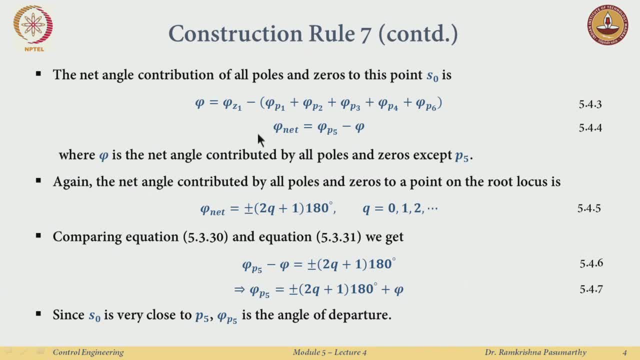 is the angle of the 0s minus all the angle of the poles, and this is how I get it and it is kind of straight forward to look at it right. And again, because you know s 0 is very close to the departure point or the pole, this will be the departure point And 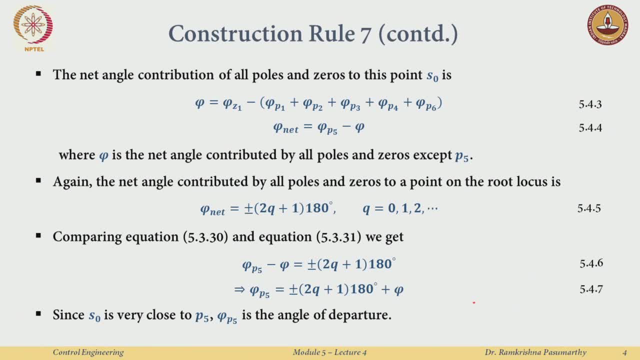 as s s naught tends to the pole p 5, well, that particular angle contribution will come 0, and then you know this, and then the other poles, or the angle contribution by the other poles, will satisfy the angle criteria. So I am not moving, I am just at that pole. 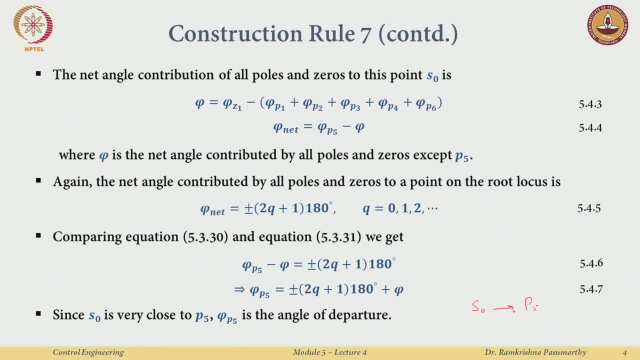 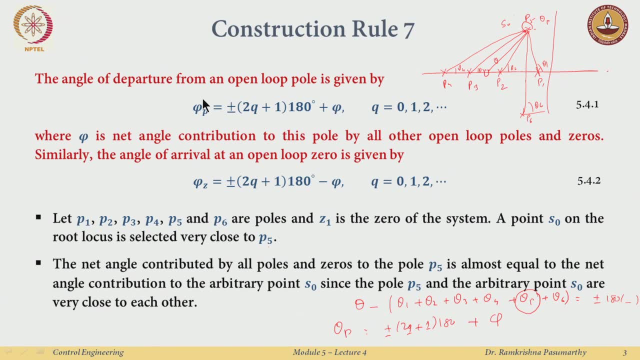 And this is the limiting condition, as s naught goes to s 5, but s naught being very close to s 5, how do I compute the angle? well, that is just by this phi over here, this guy. Similarly, I could even do for a 0, right, This is exactly the same procedure. what I would do for a 0. 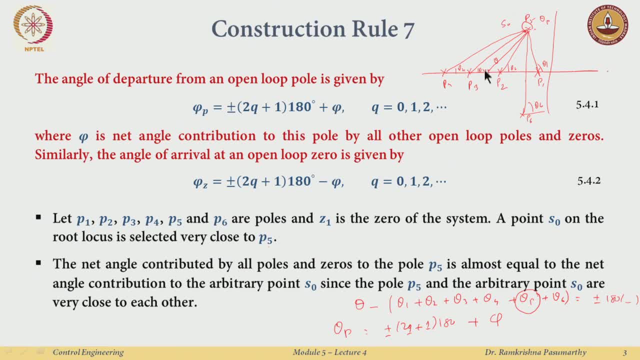 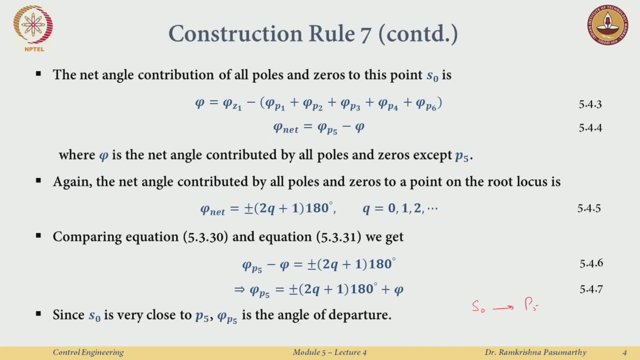 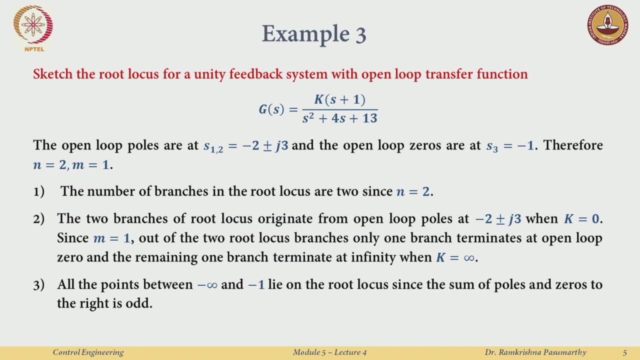 take the 0 and you can just compute. take a point, just this, to the left or right, or, you know, top or bottom of the 0, and then the angle could be computed kind of quite easily. So we do an example. sketch the root locus for a unity feedback system with open loop transfer. 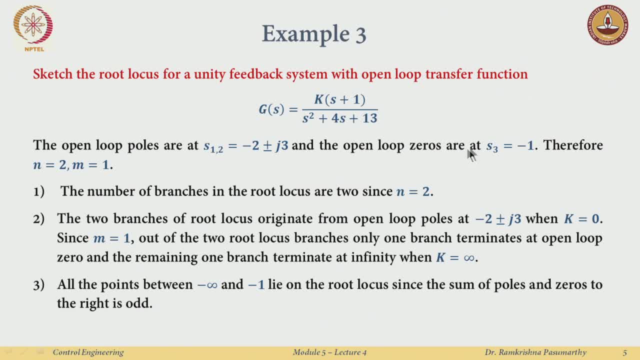 function. again. we have complex conjugate poles, open loop. this is 0 at minus 1, n, equal to 2, m, equal to 1. number of branches is 2, 1 and there is a 1- 0. So 1 pole will go to 0 and 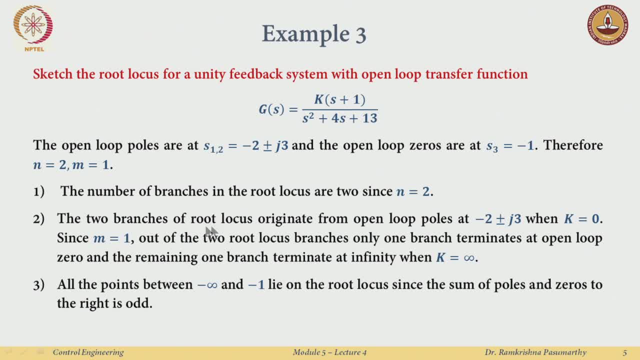 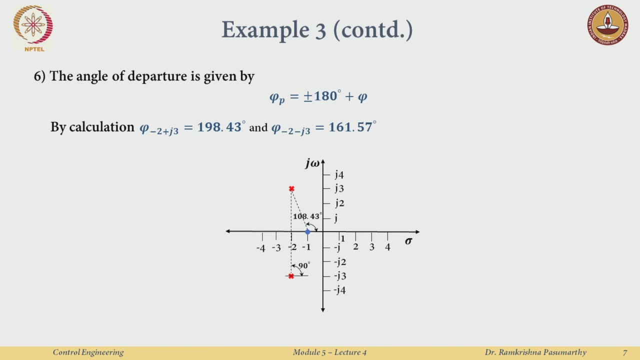 other will go to infinity. ok, And the 2 branches originate from here. when k equal to 0 and m equal to 1, one of the branches will go to this guy, another will go to infinity. ok, So let us see how the plot looks like, right? ok? So in, this is the rough sketch of it. 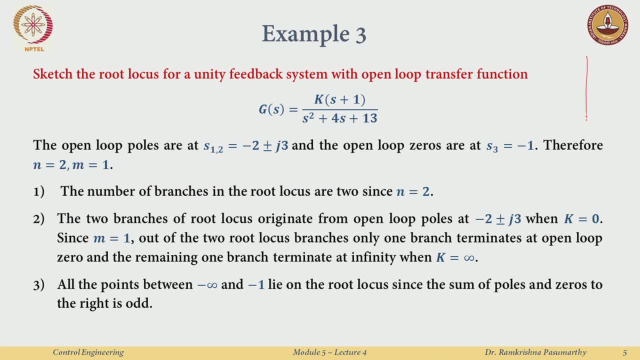 before. So this is a good space here. So I have a 0 at minus 1 and my poles are here: minus 2 plus j, 3 and minus 2 plus n, equal to 1. ok, So now this is done, we get the w. 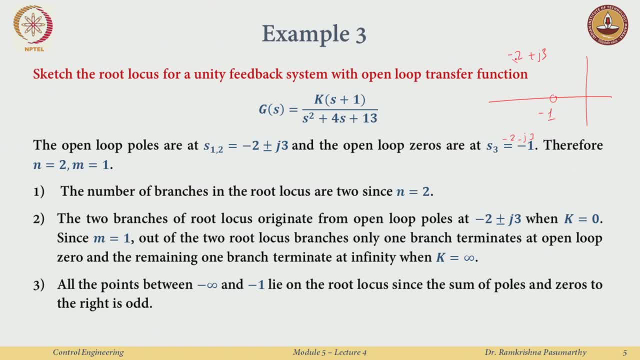 of the 10 to the power 2, one of the 10 to the power 1.. So 1 minus 1 plus 2 minus 2, 2 minus j, 3, a pole here and a pole here. So I just want to see you know which direction. 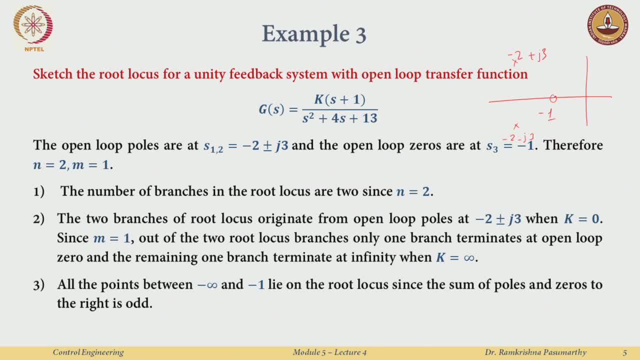 this move. but before that, well, let me do the first rules right. which point is on the real axis? I know that when I start from k equal to 0, I am here. k equal to 0, I am here. k equal to 0, I am here Now. just look at this. there is nothing here, right? So this? 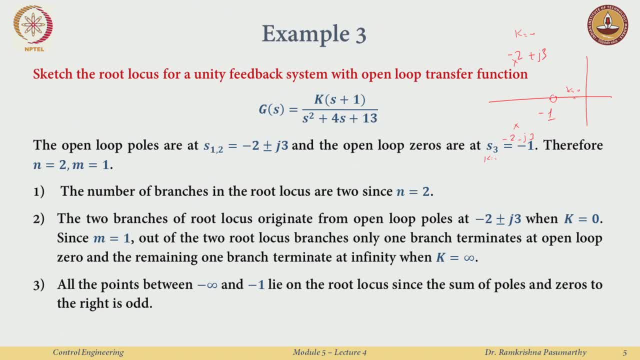 point would not, this region would not be on the root locus right. there is nothing here, and look at the point here, right. So from here I go to the left of minus 1, there is just 1, 0 odd number. then I go again here. there is again an odd number: 1, 2 and 3.. Sometimes 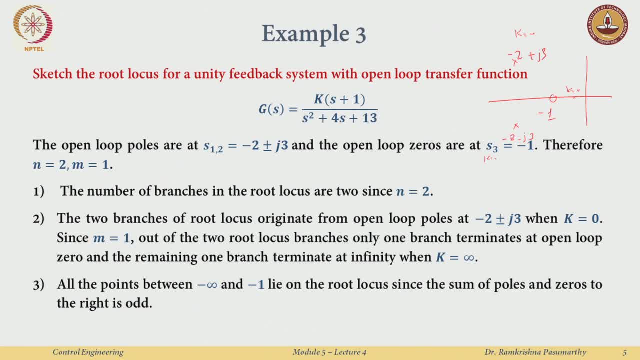 we can, even if we even neglect this complex poles for counting, because they always are in conjugate pairs, right? So there is even before this guy, there will always be an. even even after this guy, if there is an odd, there will be not. So the, at least I know that. 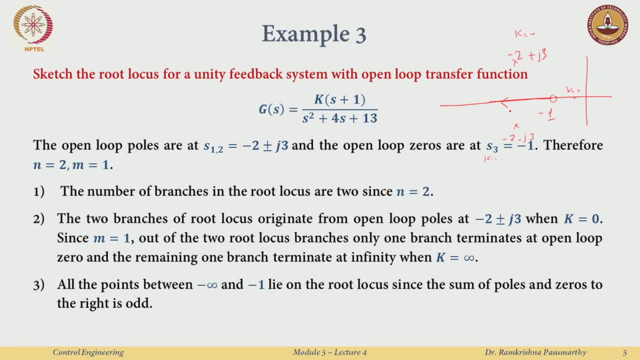 the entire. this guy is on the real axis now. is a is on the on the root locus correct? ok, I will not even draw that out. I will draw the arrow at the moment just to be a little safe. So this entire line is: 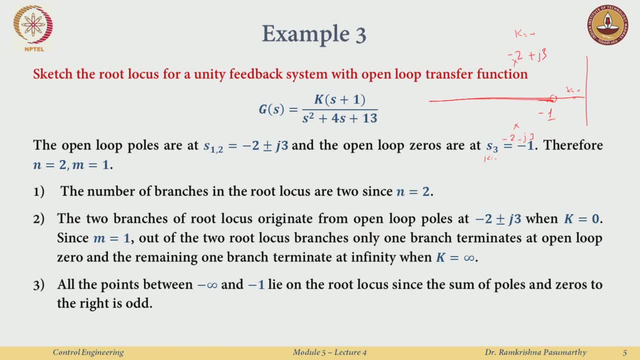 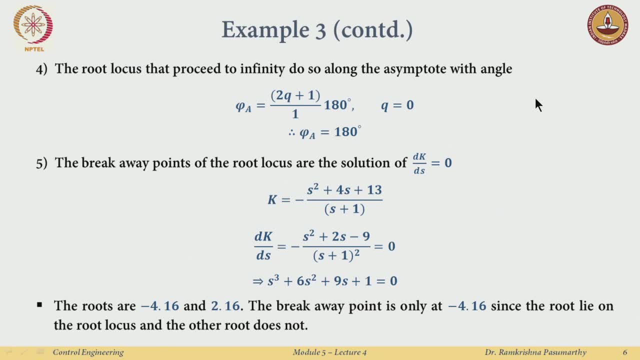 on the root locus, starting from the left of minus 1. ok, So again I do all the basic computations that well, there is one guy which goes to infinity. what is the angle which that guy goes to infinity? well, that angle is 180 degrees. 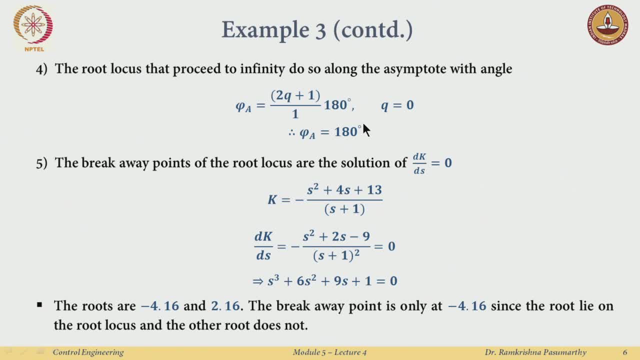 And its just very straight forward to compute: n minus m is 1, so this 5 will be 180 where? and then these guys- well, do they really meet at some point? and then go away? I can just find by dk, by ds, equal to 0. And the solutions would be this: 1 minus 4 and 2, and I do not. 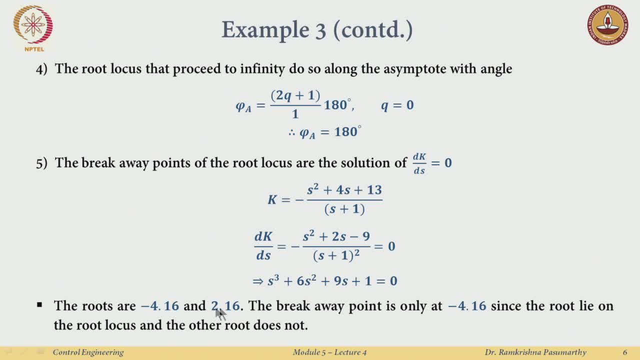 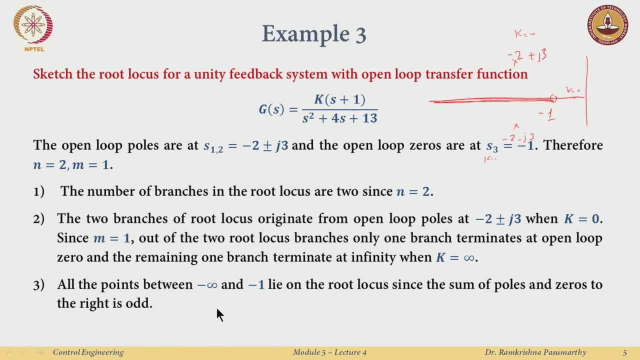 really I am not really interested in this guy, right, This is on this point does not really lie. on the root locus, I am not. I am not ignoring this because its an unstable region, right, I am just ignoring because the root locus tells me that I just cannot go. 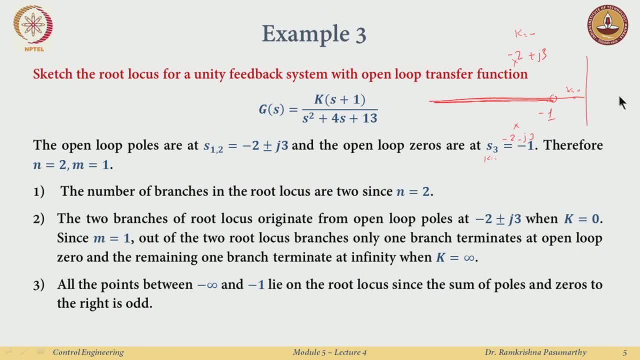 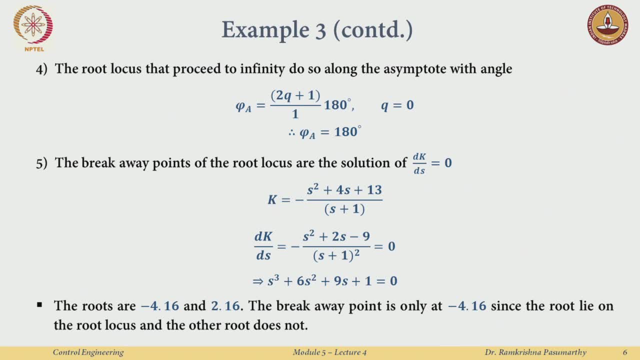 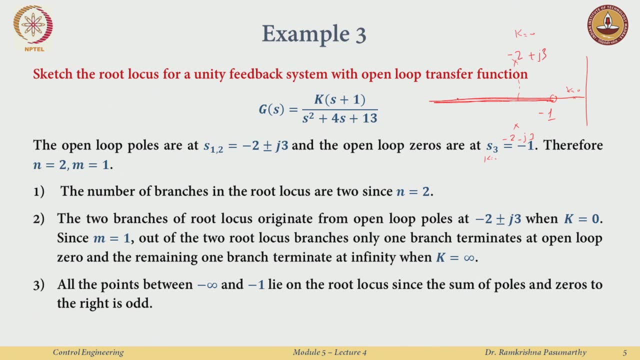 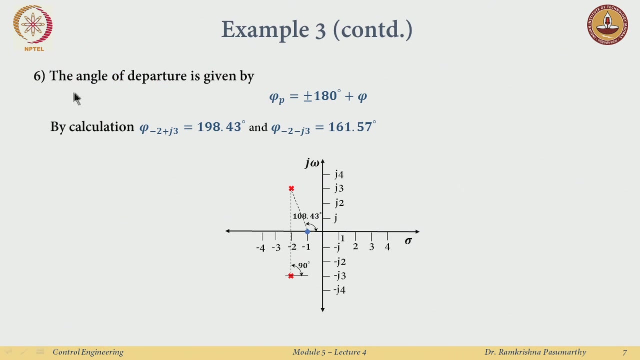 here, right, because I cannot be on any of this line because there are no poles or 0s to the right of this. ok, So I am looking at minus 4.16.. So this is real part here is minus 2, and say this is this point is minus 4.16,. ok, So I just go now to compute the 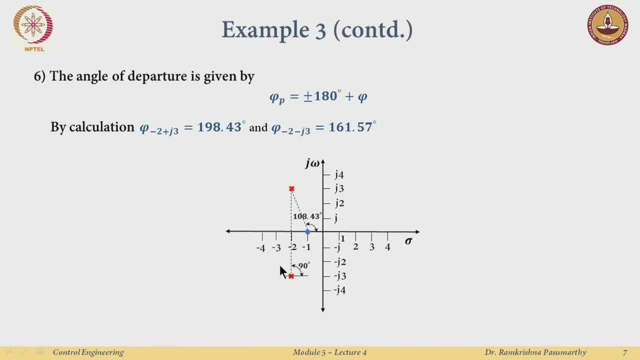 angle of departure from this side and departure from this side right. and then there is this formula: phi of p, if I am looking at this guy, would be plus minus 180, plus the contribution of the other two guys, and if I am computing phi for this guy, it would be this: phi would: 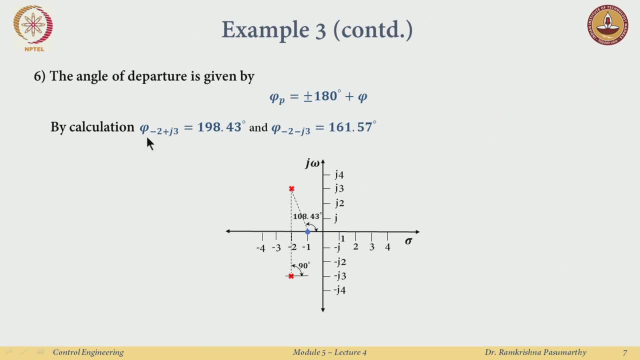 be the angle contribution of these other two guys. ok, I can just compute- this is kind of very straight forward to check- that phi for this guy would be 198 this way and phi for this guy minus 2, minus j 3, would be 165, ok. 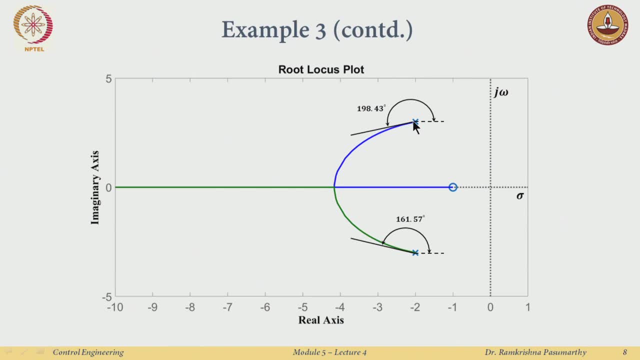 So I just know that I am just from here. sorry, I just move in this direction here, I just move in this direction. I also know where I am meeting, right at minus 4.16.. So the locus will start from here, will come here, will come here, and therefore the directions. 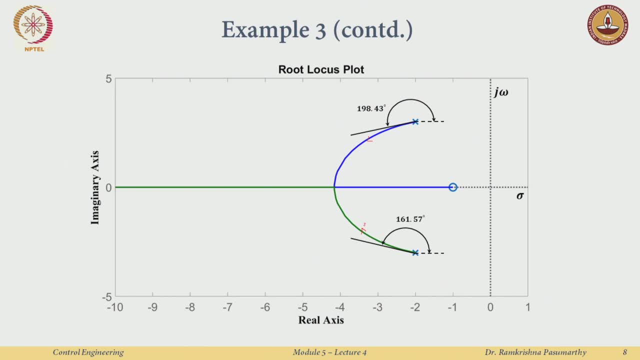 would. something will be something like this: This guy moves here, this guy moves here, this guy goes here, and this guy goes here, right. So now I know, Why is it this way? Why is it not like something like this or any other thing? Why is it not? 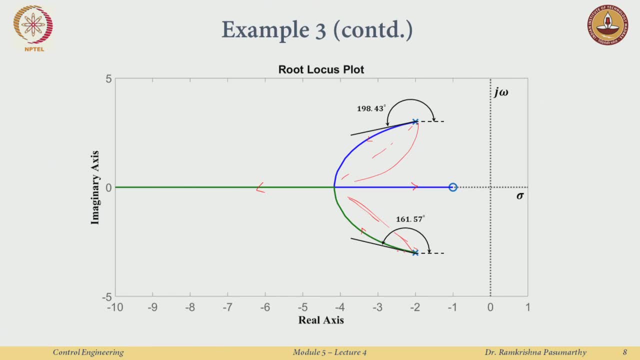 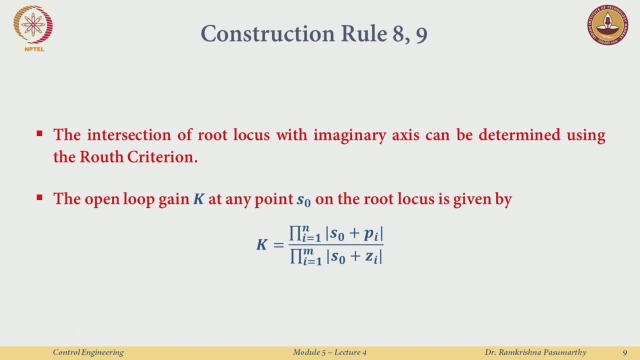 like this right. So this I just this angle tells me why, how it behaves. ok, So this is something not very surprising, this rule, How do I know if my root locus intersects with the imaginary axis? Well, when I hit the imaginary axis, say I have a root. 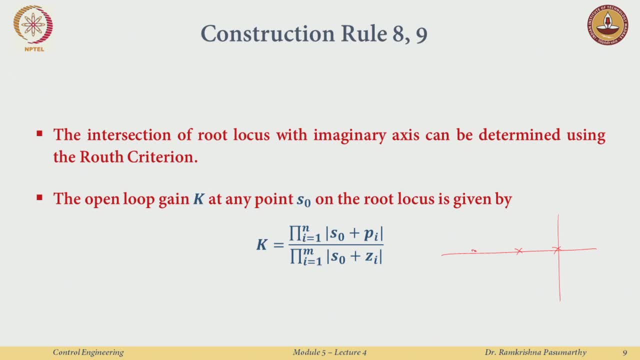 locus, which is like this: Let us say, I have three guys here and I say: well, this guy is- I am just doing an approximate plot- right? So this guy, there could be something like this, right, There could be possibilities of this thing, and these guys are going here. 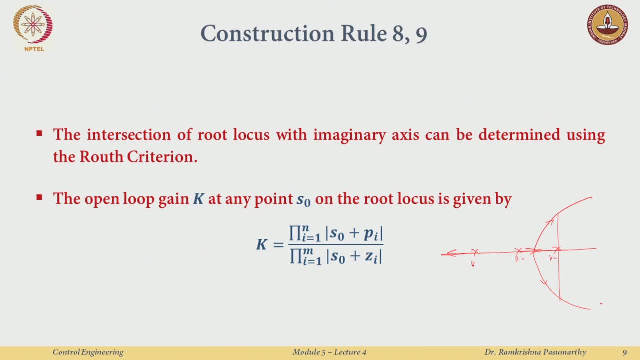 So these are all k equal to 0, k equal to 0, k equal to 0, and I see that after some values, you are actually going this side. you are going in the unstable region. Now can I really compute this value when it becomes unstable? There was a problem. There was a. 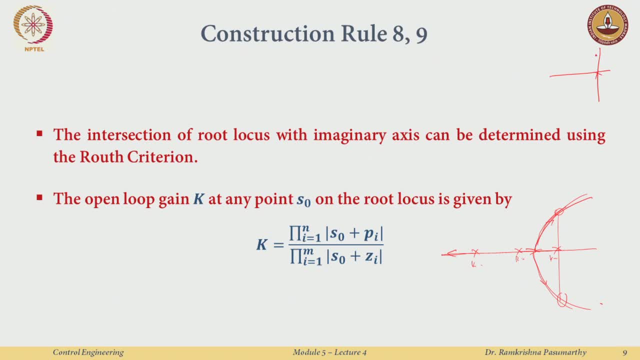 another example where my poles were here, here and here, and then the root locus: well, one guy was going this side and other, well, other two guys went here. So for any value of k greater than 0, it was always unstable. right that was. that was not difficult to compute. 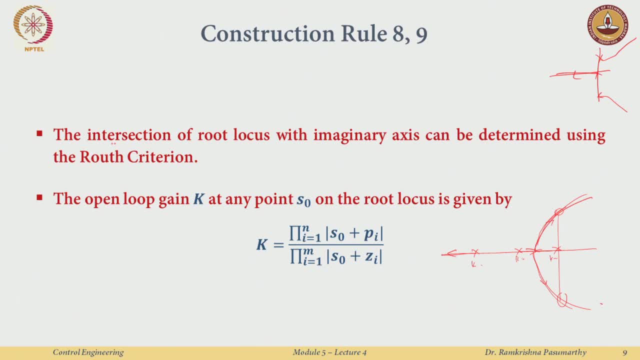 Now, how do I handle these conditions? Well, I know something called the Routh Hurwitz criterion. right, The intersection of the root locus with the imaginary axis can easily be determined by the Routh criterion. just to see how can? So so we had done some problem. 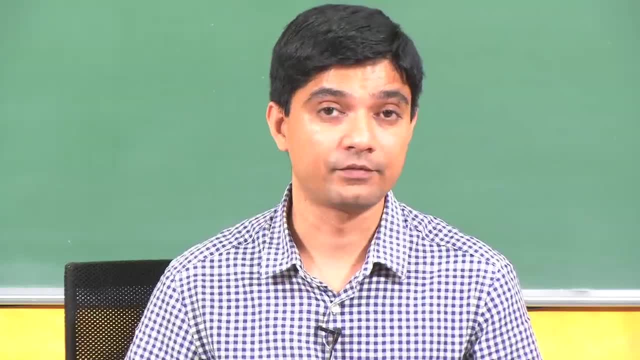 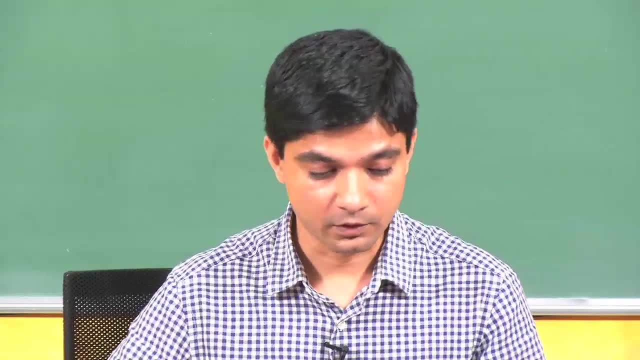 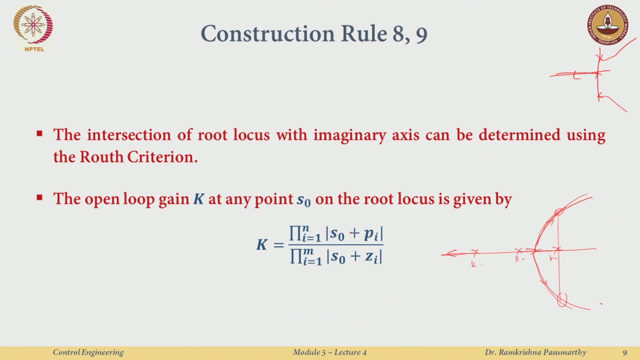 So we were computing stability with respect to a parameter, right, If k was between this number and that number, the system is stable of. if k is greater than this number, system is stable, and so on. right, ok, So, and then the open loop: gain k at any point on the root. 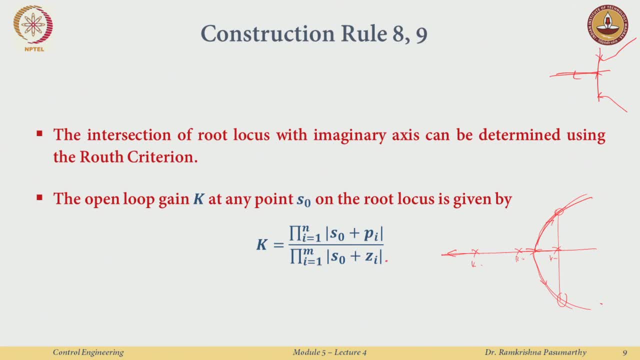 locus is just given by this. I think this we had even discussed in one of our very earlier slides. what, given a point k, how do I find the sorry? given a point on the root locus, how do I find the gain k at that point right? 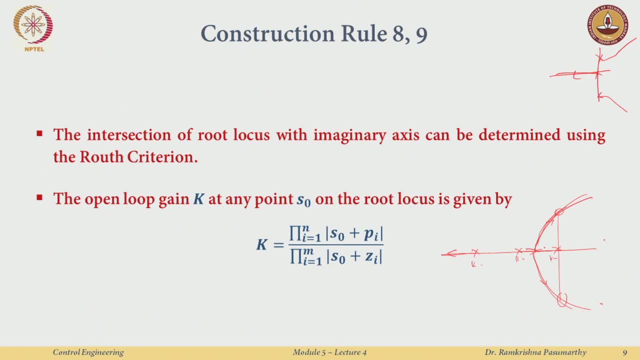 So this is just simply like this. there is nothing, nothing special here. Of course. now, if you could do in Matlab, you just move the cursor, it will actually tell you the values. but where does where does that come from? that comes from something here. ok, 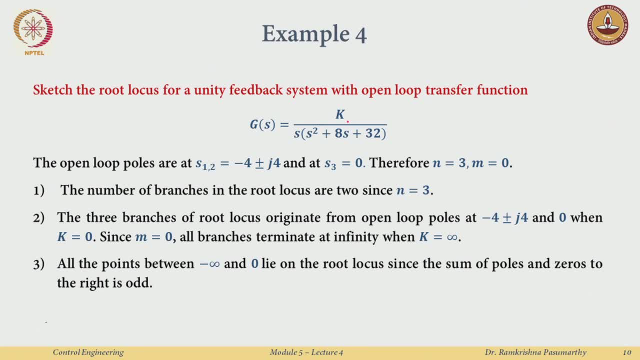 So just to do another example, So we have g of s is k. I have a pole at the origin and two other poles which are complex conjugate, minus 4, plus j, 4, and another pole at the origin. So I start from here. So I have a pole at the origin. 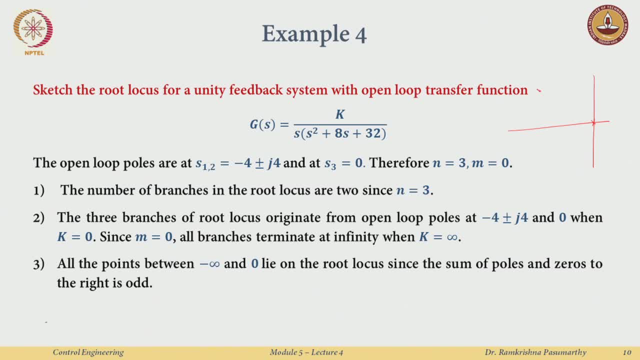 And I have two poles here. So this minus 4 plus j 4, minus 4 minus j 4, and this is the origin in the sigma and j omega axis. ok, So there are three branches, all of 3, all. 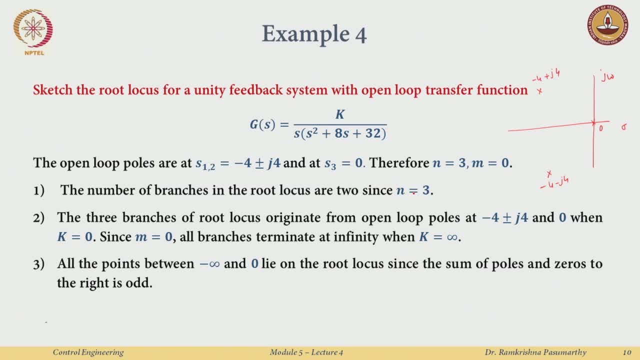 of these things will will go to infinity because there are no zeros. ok, So which points of the real line lie in the root locus? So this is fairly obvious because at any point, if I go to the left of 0, I look at to the right, there always be odd number of poles: 1 until. 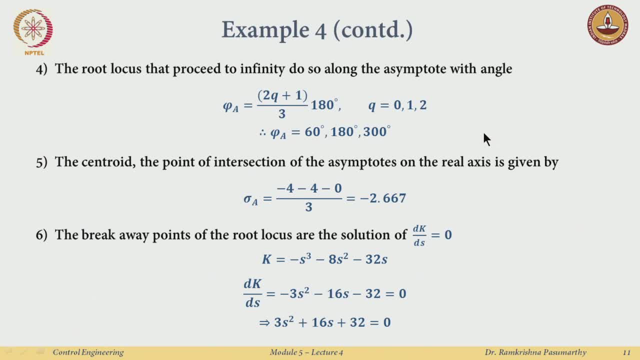 I reach here and after that there will be 3,. ok, The usual process of finding how the root locus, or how the roots, proceed to infinity. they will be at angles of asymptotes, at 60,, 180 and 300, with the standard formula, and. 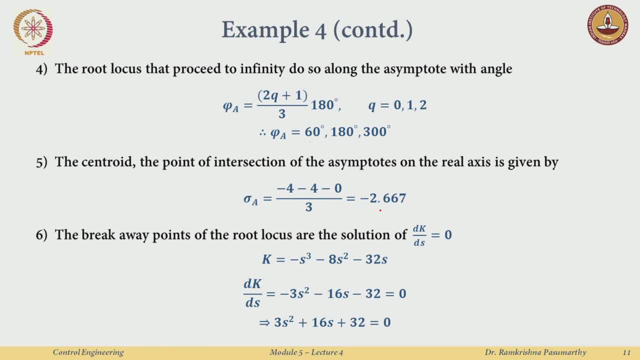 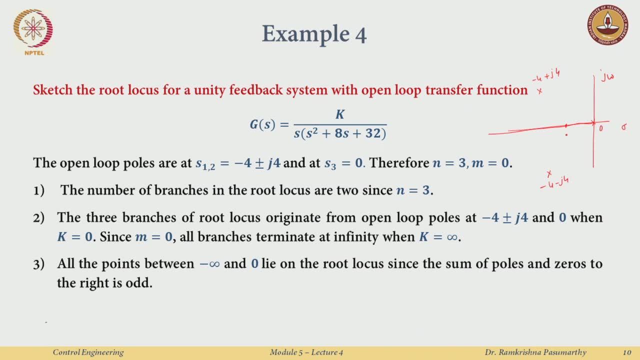 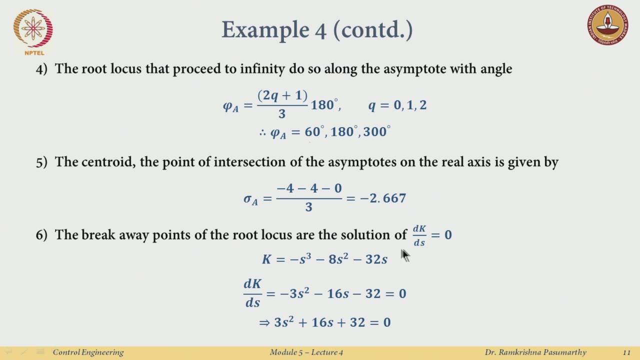 then the centroid point of this asymptotes would be minus 2.66.. So somewhere over here. So this is my sigma A. ok, So the breakaway points. well, I just look at d k by d s equal to 0, I find k and then solve for d k by d s equal to 0, which gives me the breakaway. 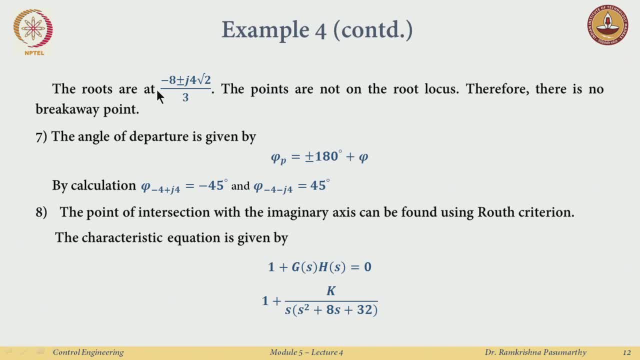 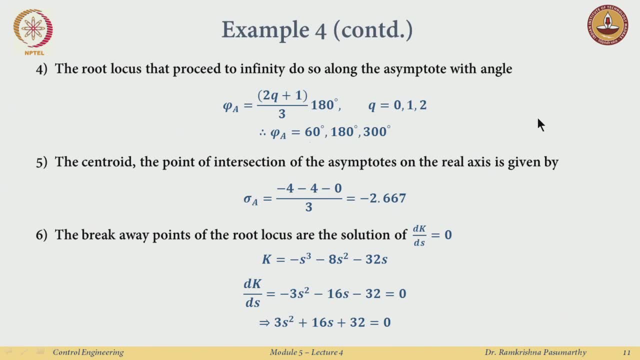 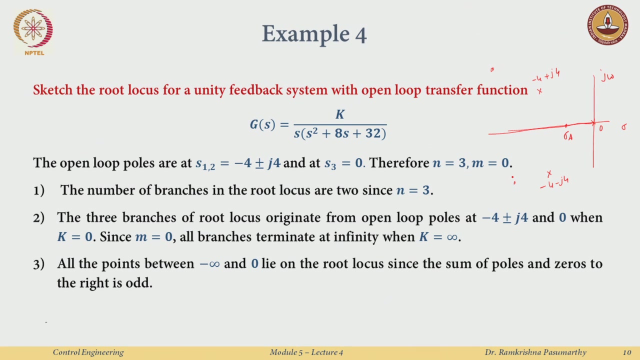 roots at this point, And I could actually see from here that these points are Very unlikely to be on the root locus, right? So say, look at this, minus 8 plus minus j, So I am somewhere here, right Then? what do my asymptotes suggest? is that, well, I am at. 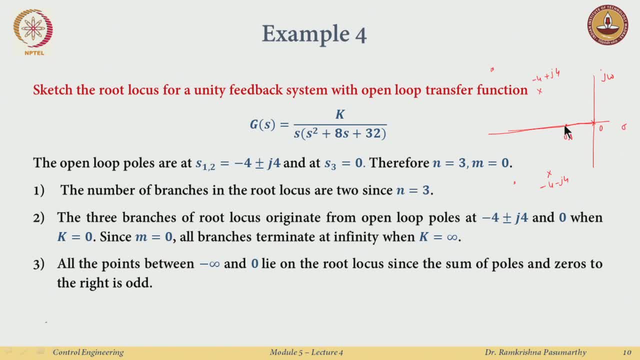 60,, 180 and 300.. So which is at an angles like over here, right? So this is where. So it shows that I should. I should actually be moving towards the asymptotes, So somewhere in this direction, somewhere. 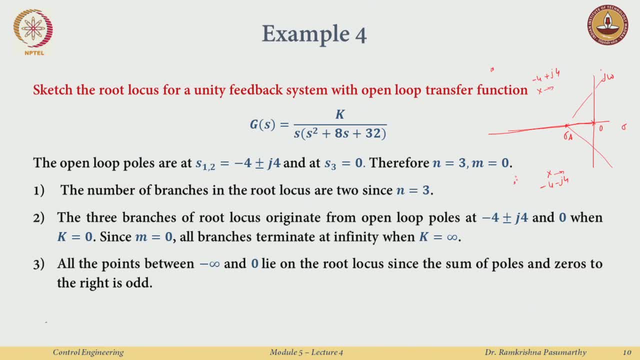 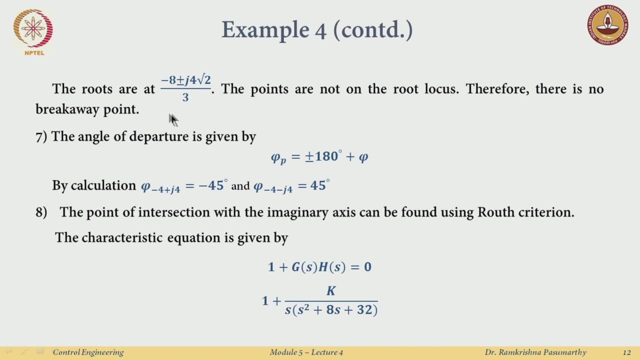 in this direction, right? So there is no way that I could reach these points based on the location of the poles, the centroid point and the asymptotes. ok, So for sure that even though d k by d s equal to 0 gives me a solution, these points will not lie on. 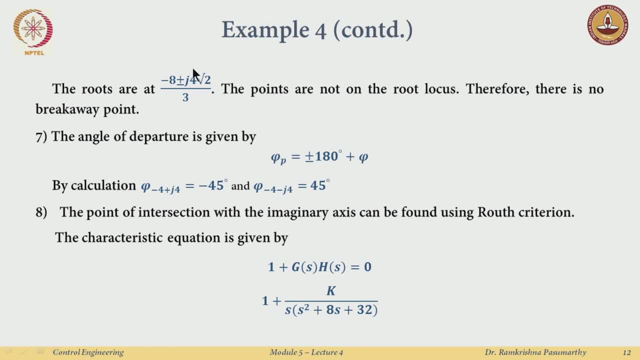 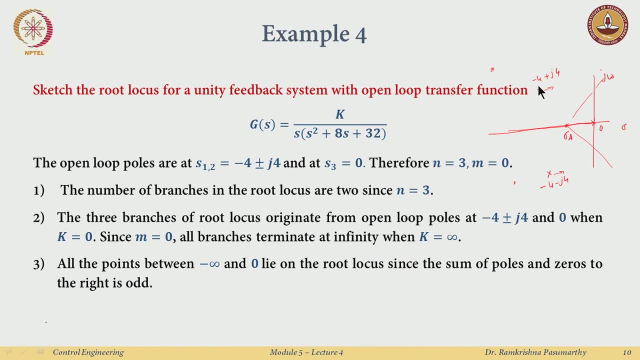 the root locus. You could also test this by the angle and the magnitude criterion. ok, Now I am looking at. I am looking at the angle of departure at these guys. So angle of departure would be computed by. you know this angle and this angle, So that should be straight forward. 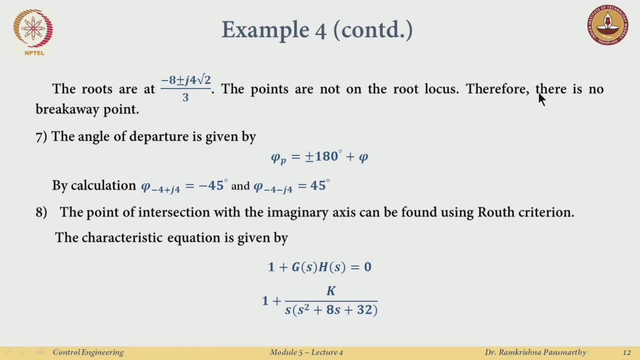 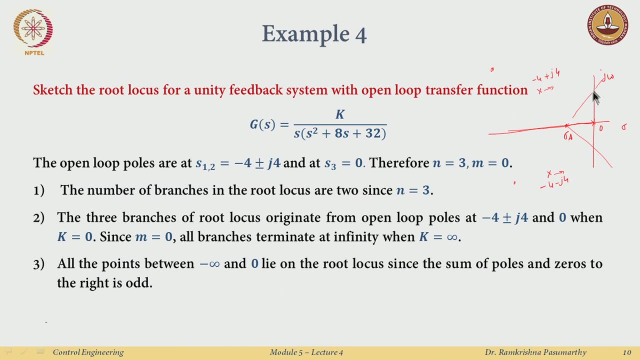 to compute. So this angle would be the angle at minus 4. plus j 4 would be 45, and minus 4 j 4 would be plus 45,. ok, Now, since these are moving in this direction and the asymptotes 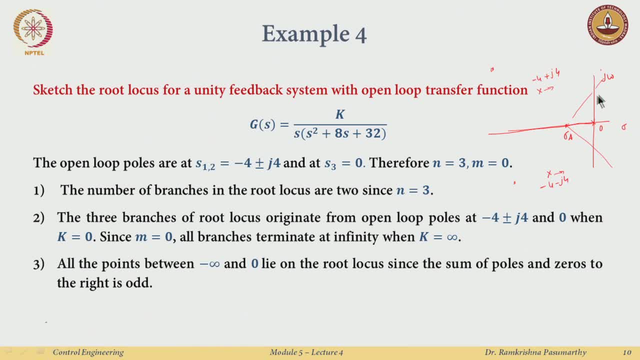 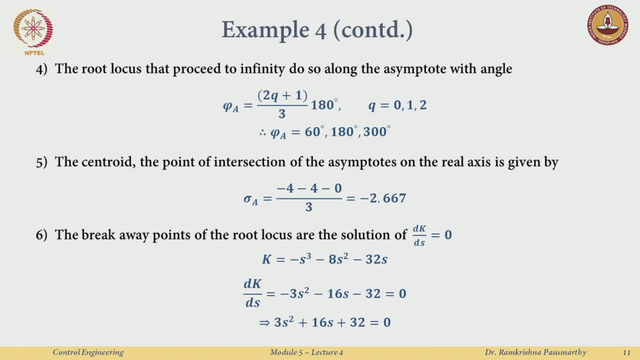 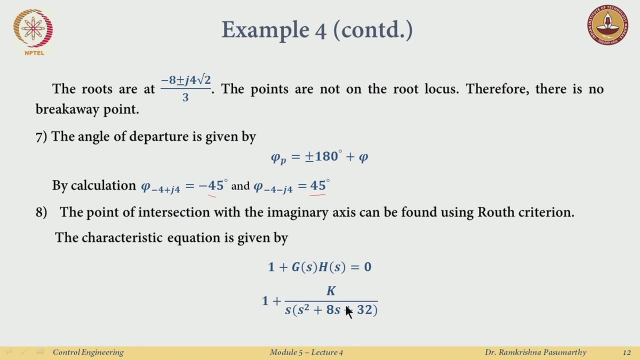 are Moving towards the right of the imaginary axis. there could be chances of these guys meeting the imaginary axis, So let us see if that is true. ok, So I write down the characteristic equation and I have 1 plus k, s, s square, plus 8, s plus 32 and I draw the. 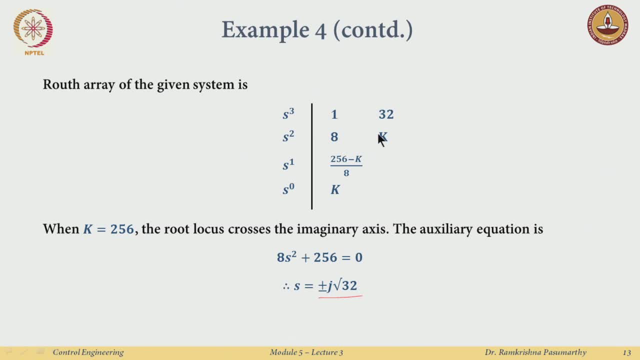 Routh table. So 1,, 32,, 8, k, this would be 8 minus 8, 8 times 32 minus k by 8,. ok, So what happens when, say, when does this guy go to 0?? This guy will go to 0 when 256 by 8 minus. 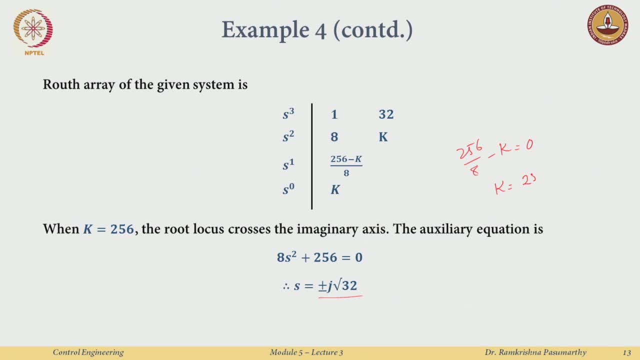 k equal to 0, or for a value of gain k equal to 256, I have this entire row equal to 0,. ok, Now let us see how the auxiliary equation looks like. So I have 8 s square plus k equal to 0, or 8 s square plus 256 equal to 0, this 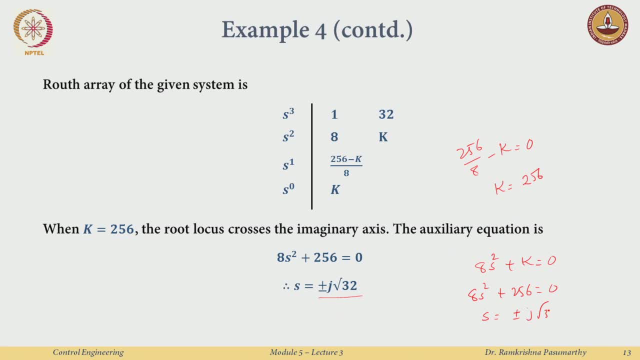 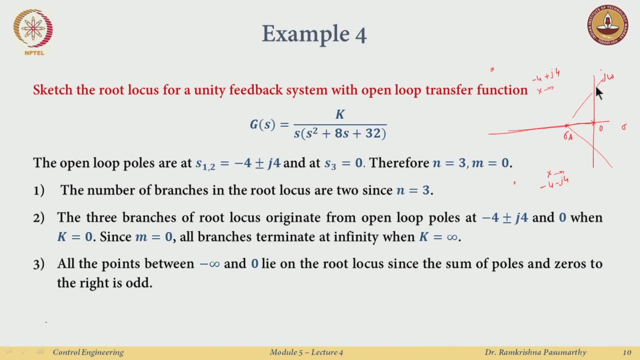 gives me s equal to plus minus j, square root of 32, and this is the value of omega, where it will cross the imaginary axis. So this will be at somewhere here: square root of 32 in the positive direction. square root of 32 in the negative direction, right? So this? 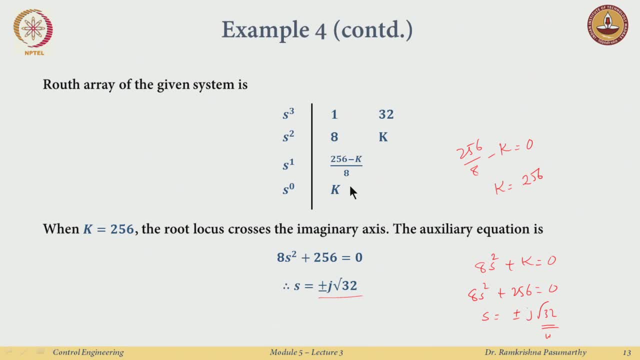 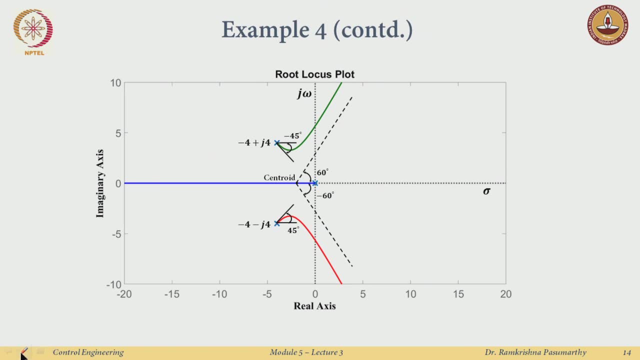 gives me a lot of information. now that there are no breakaway points, the root locus will actually cross the imaginary axis and it will actually do it this way, right? So the angle of Adventure was minus 45. So it will. it will initially tend to. 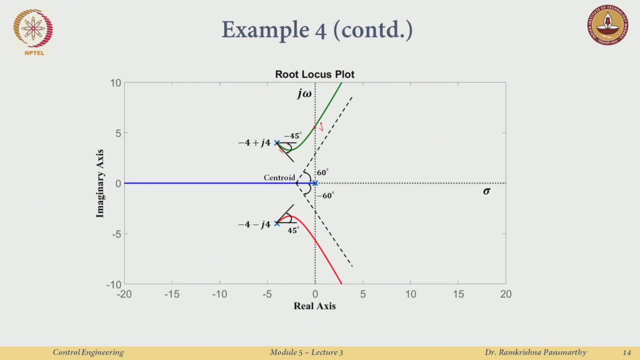 move this way, and this is square root of 32 on the j axis, and then it will just assume to this way. Similarly, this guy has an angle of departure of plus 45. So it will move this direction and it will cross the imaginary axis at square root of minus 30, sorry, minus. 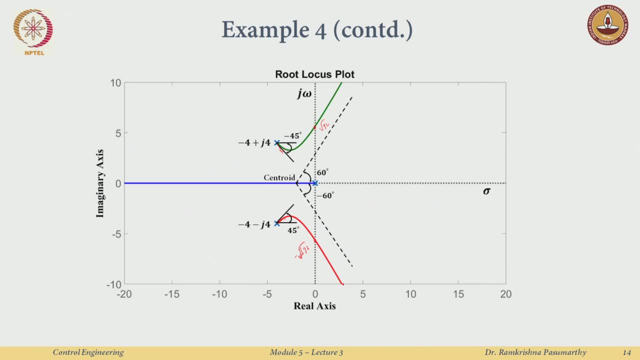 of square root of 32 and I will just do this one right. So we saw few possibilities here. right that there are no breakaway points, even though d k by d s gives me a solution. Second is to explicitly: